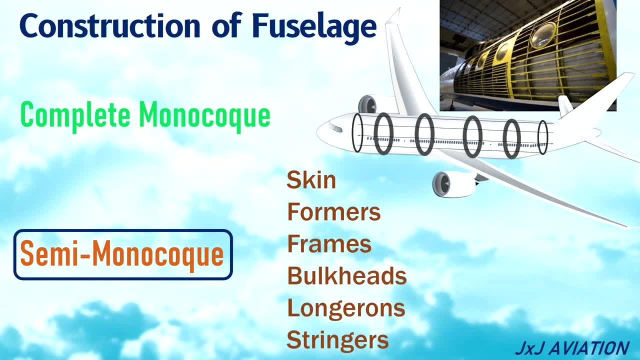 members called longerons and stringers. Here the skin is not the primary load carrying member. The load gets distributed to these different structural components. Construction of a fuselage: Most modern aircraft have a semi-monocoque type of fuselage, since it is a failsafe design. 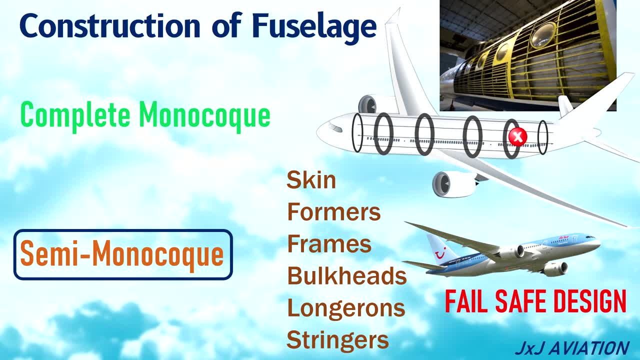 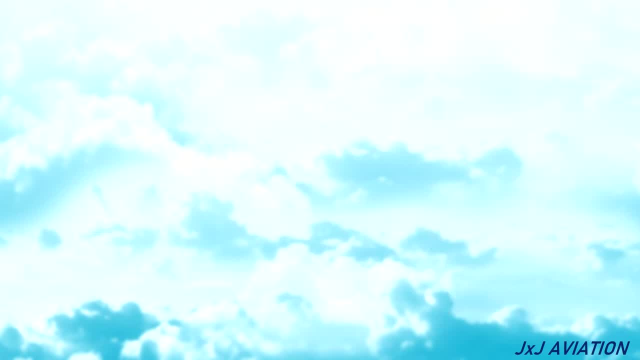 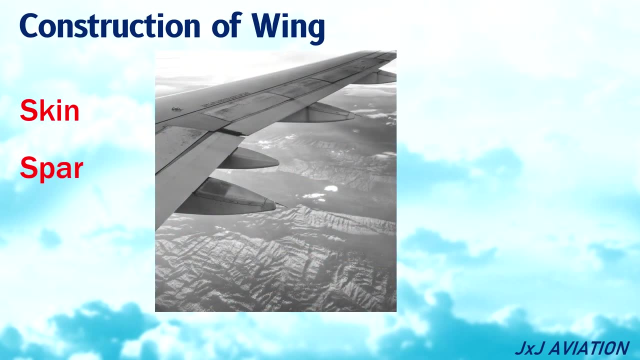 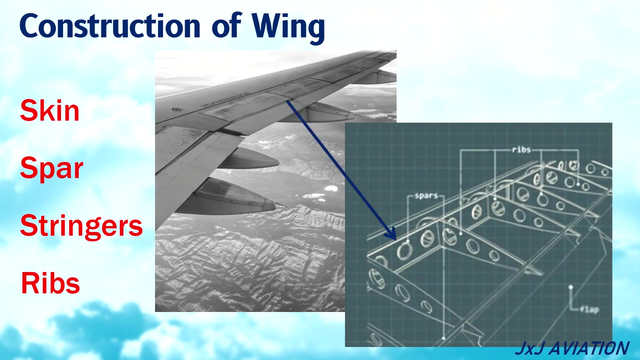 This means that failure of a single structural component will not have an impact on the safety of the fuselage. Construction of the wing: A wing is built using metallic skin, spar stringers and ribs In the big guy video will be the basic concept of fuselage. 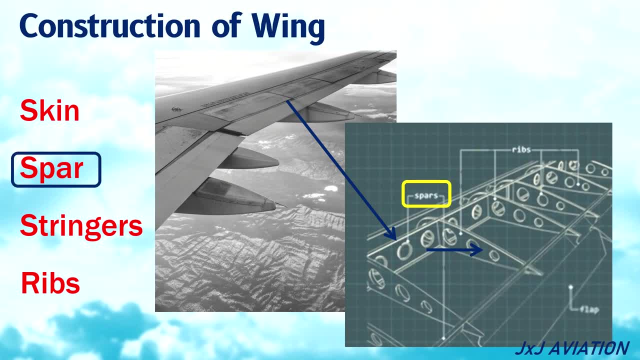 The main members of the fuselage are either row or spindle, oroffs, titties or ribs. The fields are got together using rivets or bolts. The loads acting on the wing are transmitted from the skin to the spars and the ribs. so 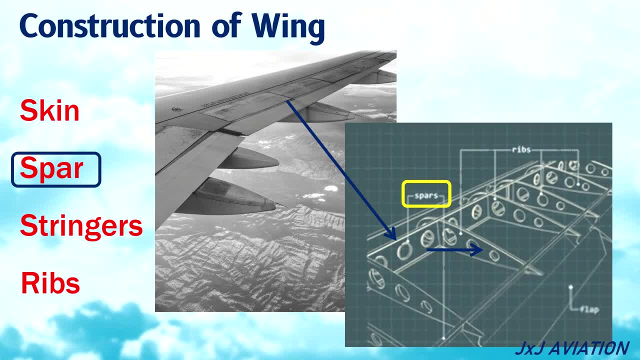 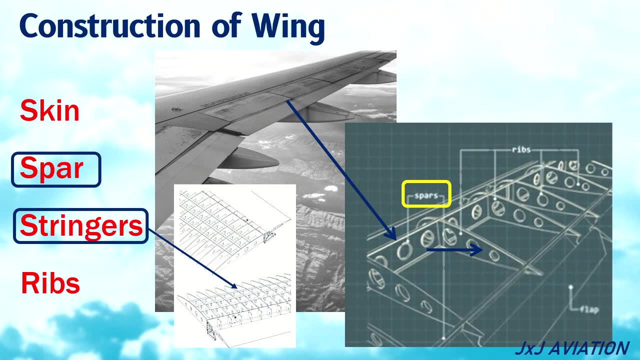 from the fuselage to the wingtips. The stringers also run along the wingspan but are smaller than the spars. Depending on the size of the wing, there may be a single spar or multiple spars used to support the wing. The ribs extend from the wing's leading edge to the trailing edge. 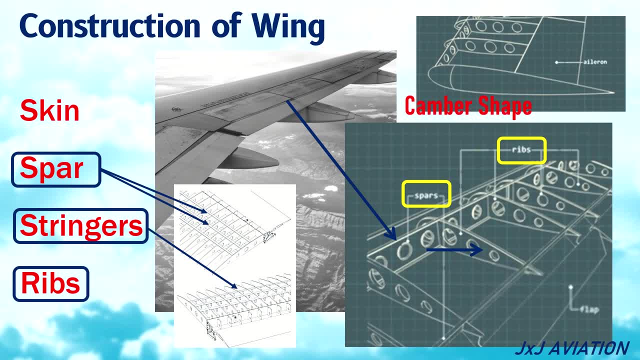 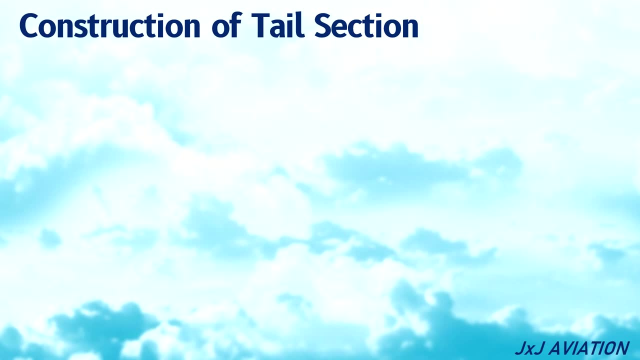 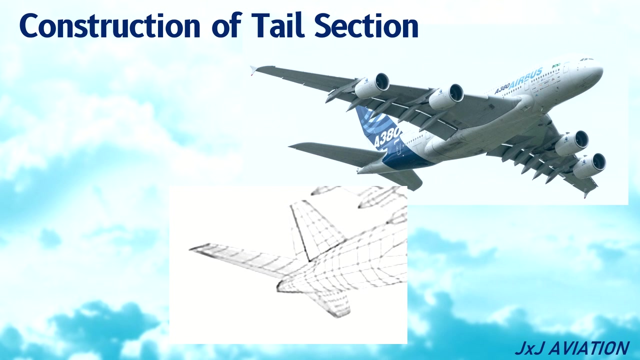 The ribs give the wing the required cambered shape and also assist in transmitting the loads to the different structural members. Construction of the tail section. The structural members of the tail section, or the empennage, are same as that of the fuselage and the wing. 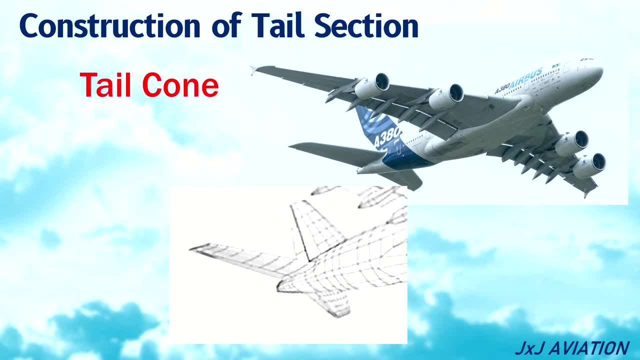 The construction of the tail cone is similar to that of the fuselage. The fuselage has bulkheads, longerons, stringers and a metallic skin. However, lighter materials are used, since less stresses are acting here. The horizontal and vertical stabilizers are similar in construction to the wing, with spars.